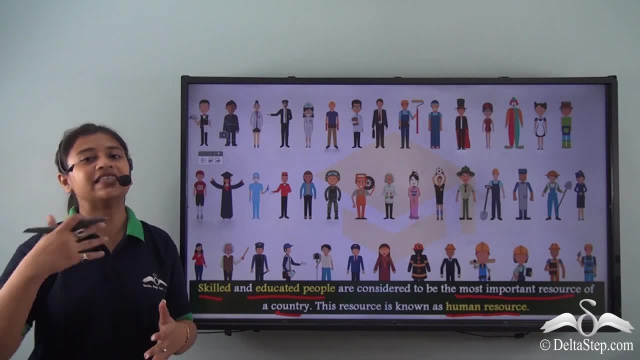 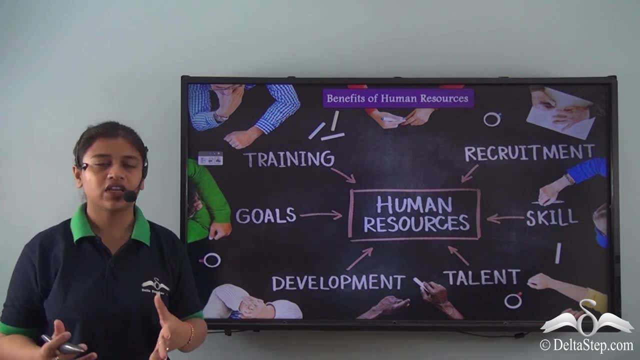 of the country. It can turn a developing country into a developed country very soon. So why is the human resource of a country so important? So human resource ensures a continuous supply of labour to the country. Now this continuous supply of labour, or people who are skilled and who are professionals at their respective fields- can lead to a lot. 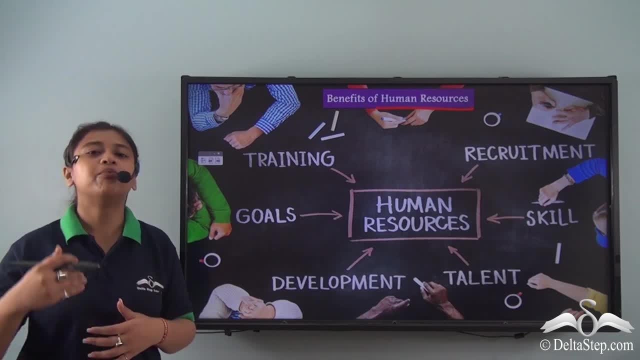 of benefits. Now. these benefits may include the boosting of the economy, the increase in the diversity of the country and thus can be very, very useful for any country. So human resource of the country is one of the most important resources that the country owns. 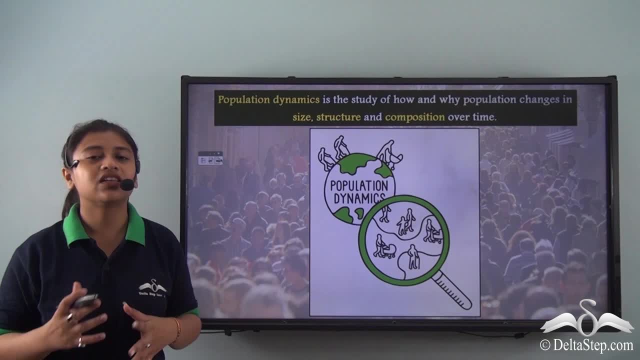 So till now we have understood what is population, The total number of people in the country, The total number of people in the country, The total number of people living in an area. and then we further understood that among the population, people who are skilled and who are professionals can be very beneficial. 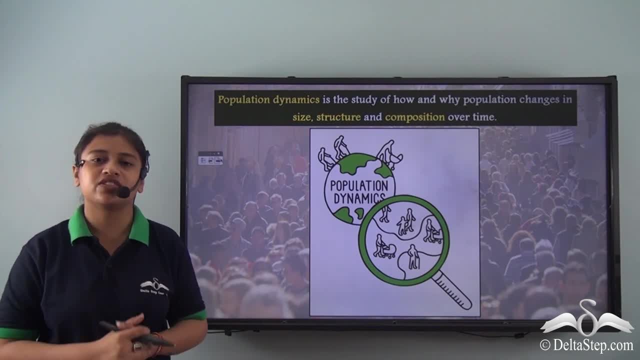 for the country or that particular area, and they are known as human resource. Now you must be thinking: why exactly are we studying population? Why is the study of population important? Well, the study of population is important because population is ever changing right, It is not static, It is dynamic. 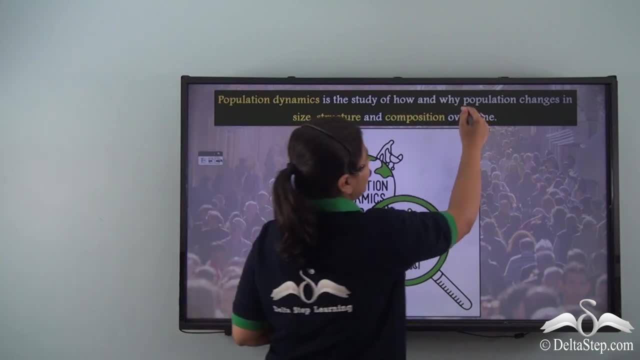 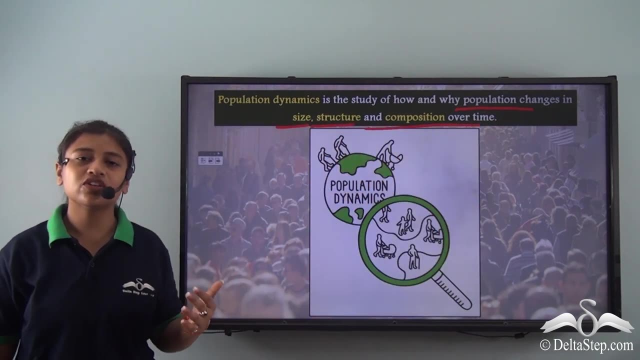 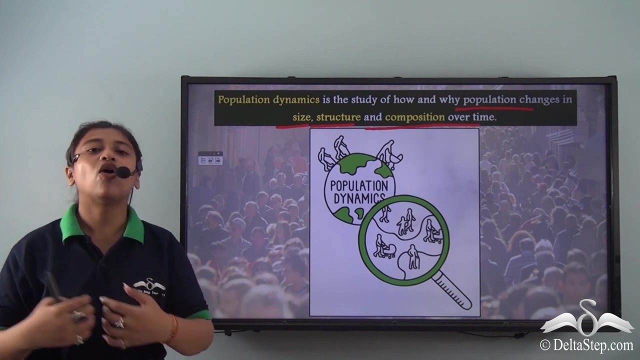 So the study of the change in population, the change in the size, the structure and the composition over time is very important so that the country can work on its people, can work for its people, for the better development or for future developments. So population: 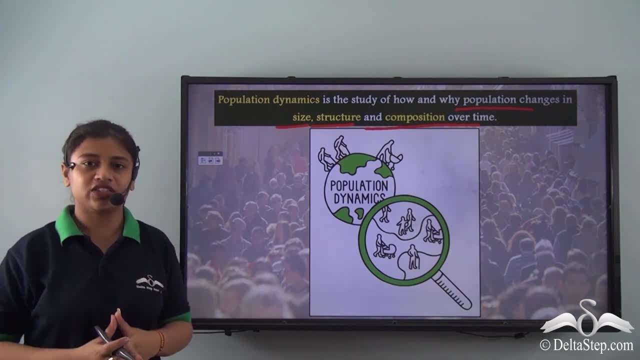 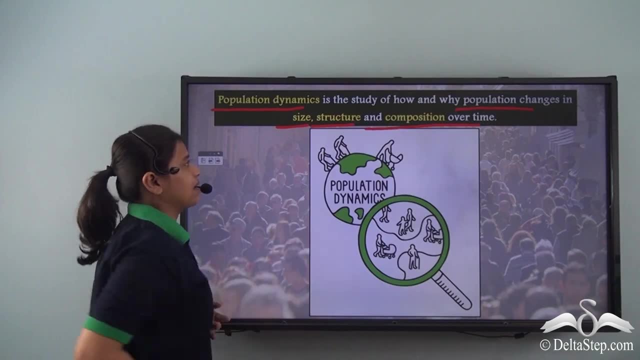 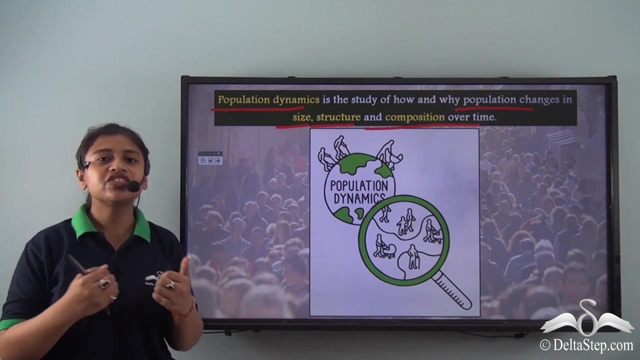 dynamics is the study of the change in population, of the size, structure and composition of population over time. so this is what is population dynamics now, the study of population dynamics helps the country understand the needs of the people, the interest groups, and what exactly the country needs to focus on so that they are not lagging behind and so that their development is not. 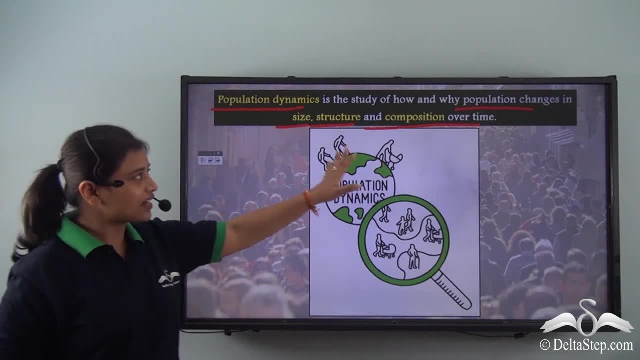 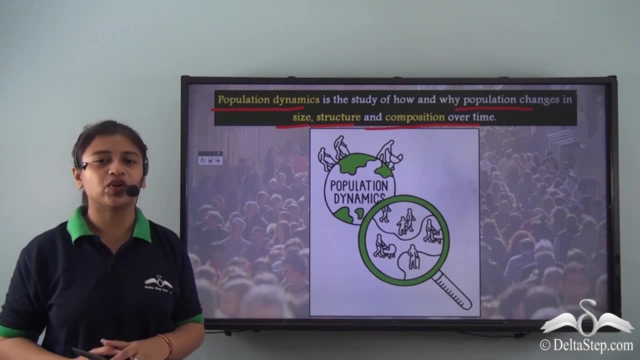 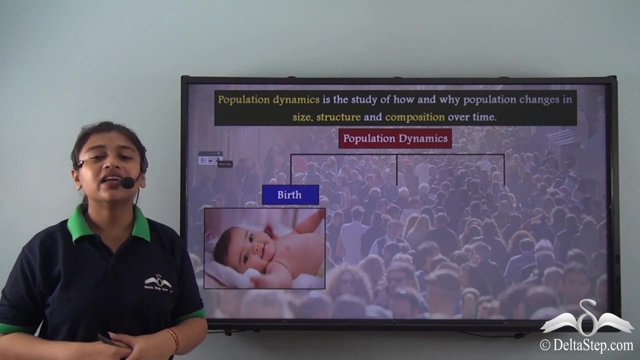 held back. so population dynamics is the study of how and why population is changing in size, structure and composition over time. now, now there are various reasons why the population changes and how it changes. right so, as and when a baby is born to a mother, it means that the population of that 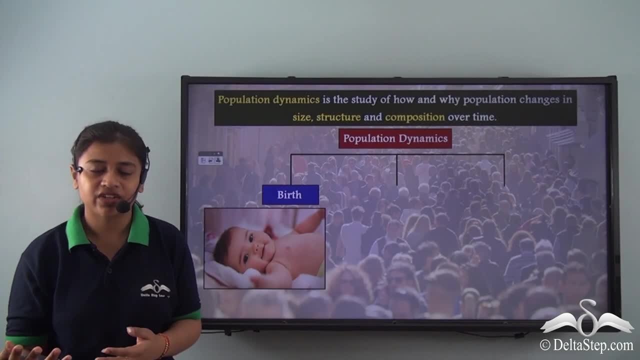 particular area where the baby is born, it has changed, which only means that each birth leads to the change in the size of the population in a particular area. but we must not forget that, on one hand, where there are births taking place, there are also people dying, on the other hand, due to various reasons. so, on one hand, where births can, 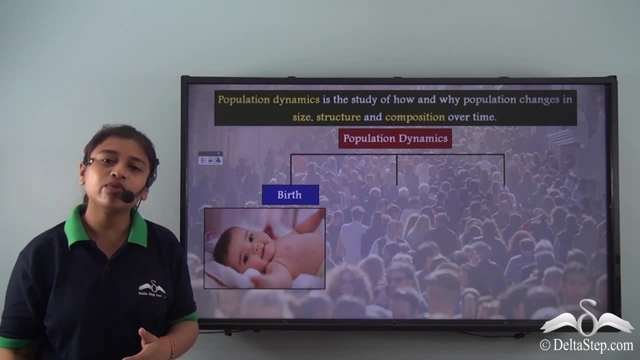 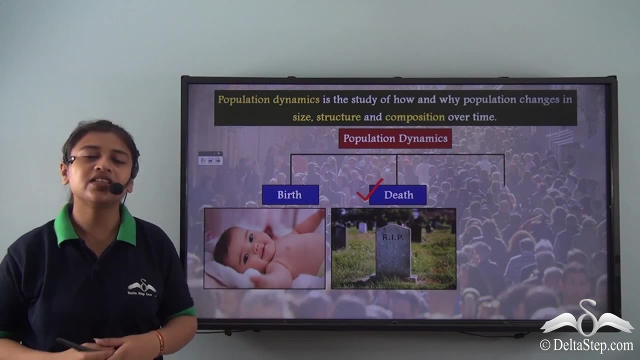 change the size of the population or it can influence population. on the other hand, even deaths can influence population of a particular area. so we can say that birth and death are involved anywhere in the population, where each birth of each population. you may, Рuby, thank you, remember to move your mouse while reading the citations. now, number 12 is not the answer. what is the size and value of the population? commenln? so raise your hand in the comment section. you have a question. if you can, you can also put the inner Quit option, the button so that we can bring the answer back to the question next opens up. so we canismo今天oms. 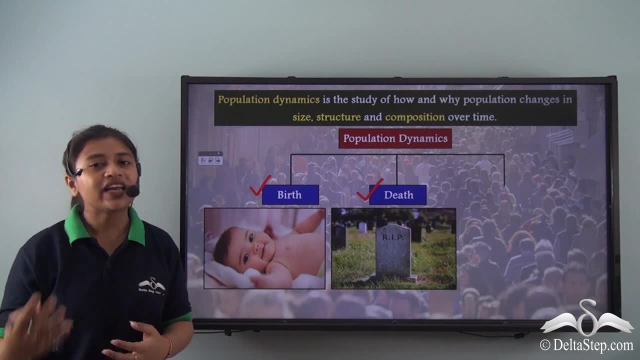 important factors or determinants that lead to the change in the size, structure and composition of a population. However, we must not forget that population dynamics does not only include the factors like births and deaths, but it also includes migration. How is that So, as 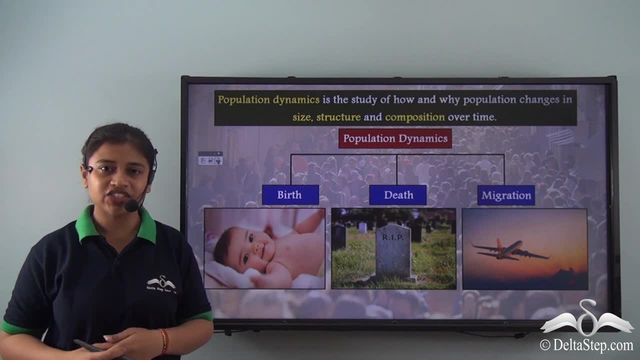 we have studied already in our previous lessons of migration that migration is the movement of people from one place to another to live in a new location, either permanently or for a short period of time. Now, if you wish to revise the chapter on migration, then you can. 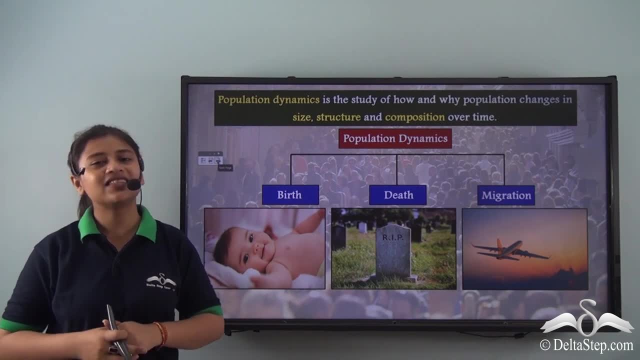 simply click on the iDictionary feature and revise the lessons accordingly. So migration is therefore the movement of people from one place to another. So if people are moving out of a country or they are moving into a country, which only means that they are changing the composition, 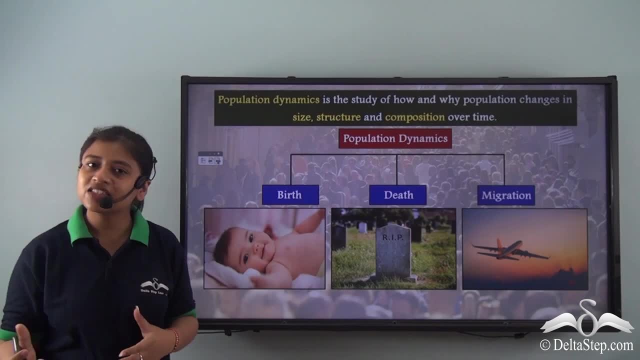 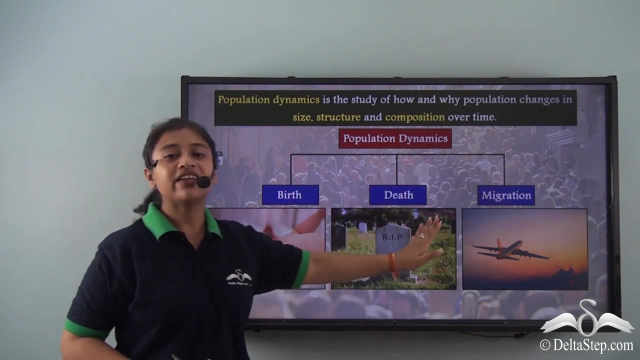 The size and structure of the population. So they are either decreasing the population or increasing the population, or they are either changing the composition, as there are different people from different places coming into the country or going out of the country. right, So we can say that these three factors- birth, death and migration- are important determinants. 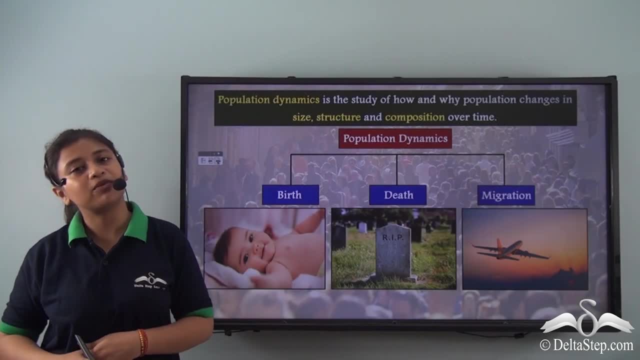 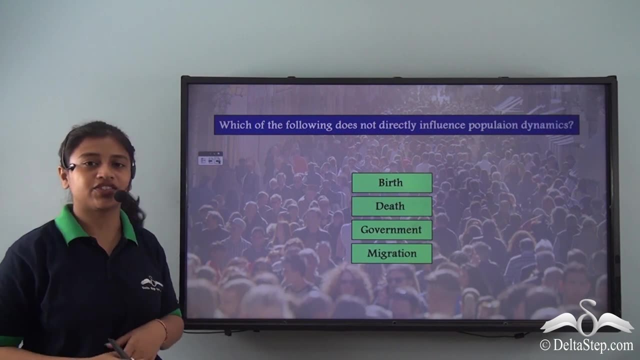 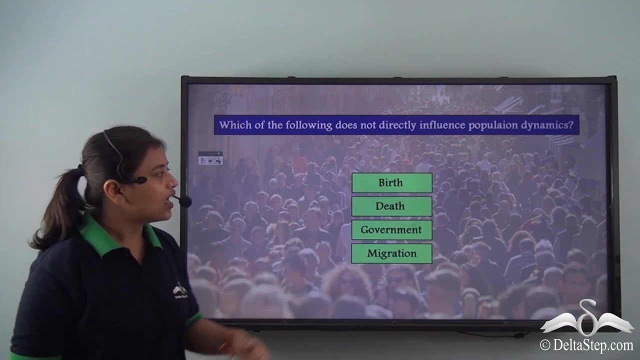 that helps in the change of size, structure and composition of a population. So before we proceed with our lesson, could you help me answer this question? Which of the following does not directly influence population dynamics? Is it birth death seth? 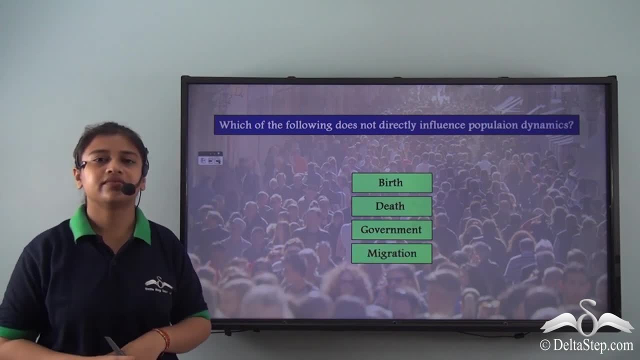 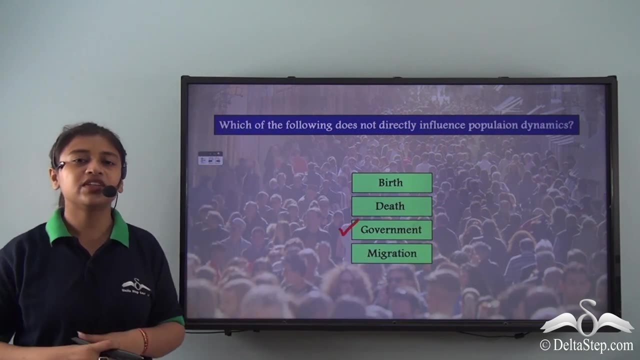 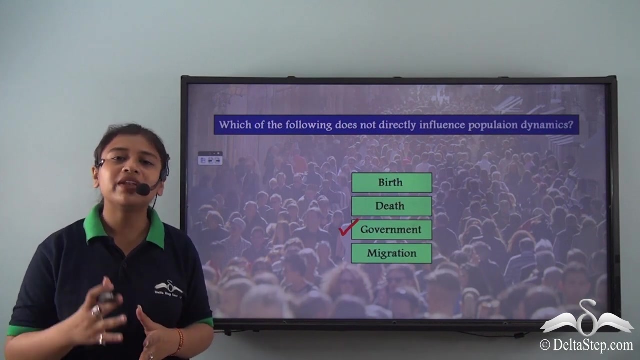 government or migration? Yes, The correct answer is government. Now you might be confused that why does the government not influence population dynamicsNo, it's not that Government influence population dynamics, but it does this indirectly and over a certain period of time. that is, it does influence the change in the size, structure and composition of the 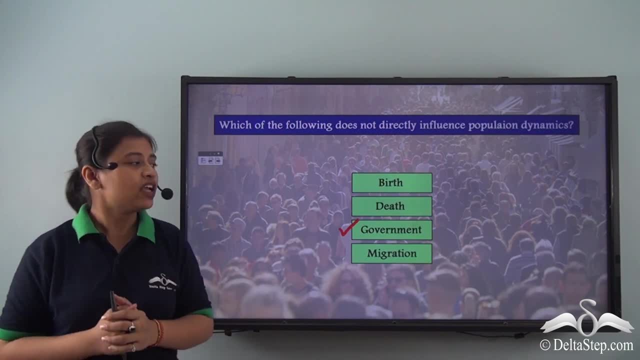 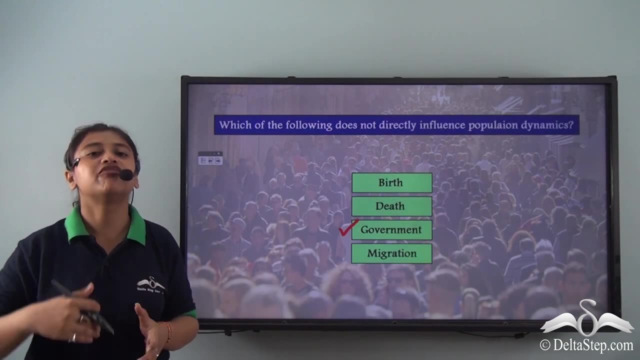 population, but gradually and not immediately. So we can say that while birth, death and migration are immediate causes, that helps in the change in population or influences population dynamics, that it directly influences population dynamics. government does not directly influence population dynamics but it does that indirectly through its various programs. 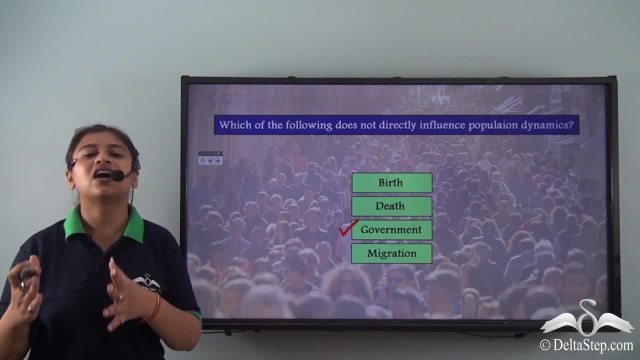 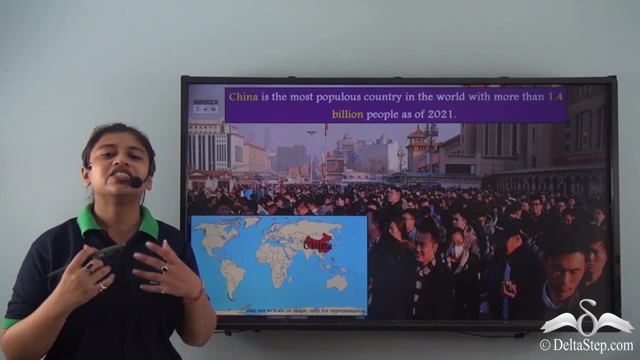 policies, its administration and various other such things. So the correct answer here is government. So we just understood that the world is densely populated, though there is a decline in the growth of population expansion since the 1960s. However, there are regions who are very densely populated. Now let's see which is the most densely populated place in the world. Now, let's see which is the most densely populated place in the world. Now, let's see which is the most densely populated place in the world. Now, let's see which is the most densely 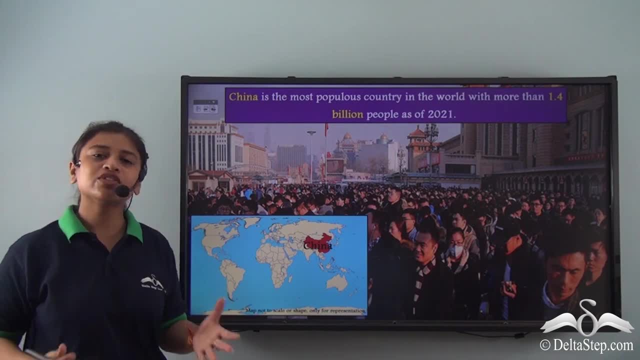 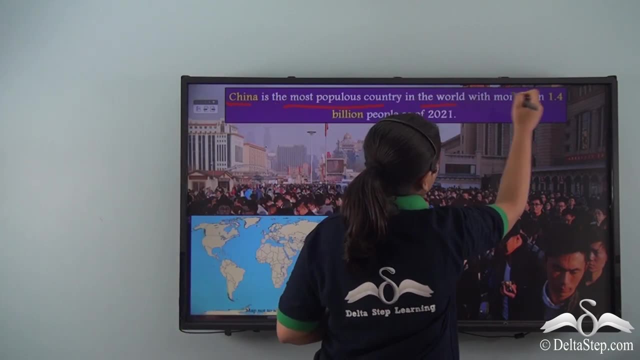 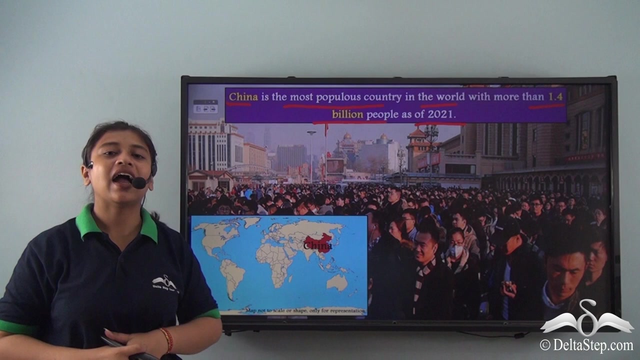 populated country of the world. well, I know that most of us here already have an idea that China is the most populous country in the world, with more than 1.4 billion people as of 2021. so here we have China, and it is said to be the most populous country in the. 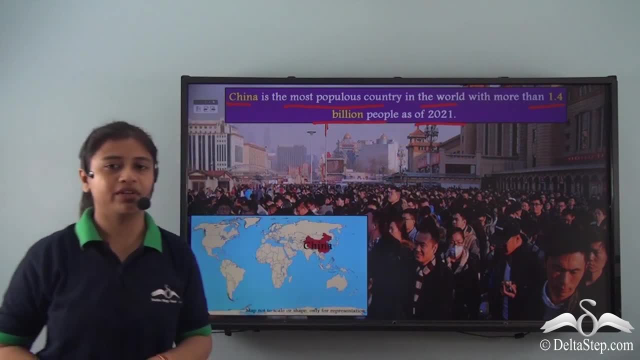 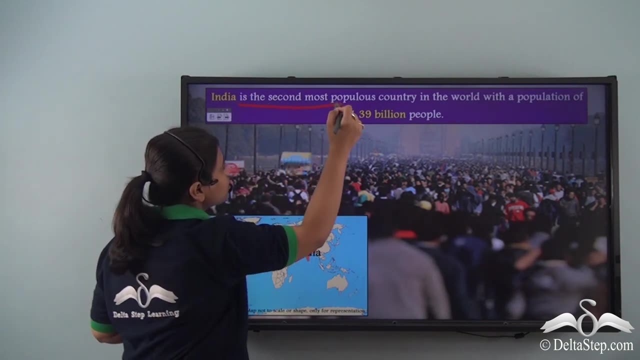 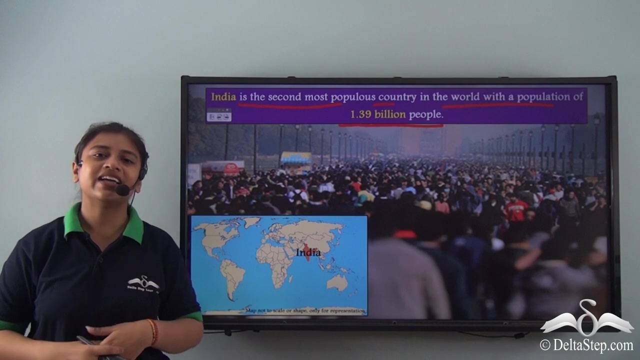 world with a population of 1.4 billion people. now, India is not too far. India is the second most populous country in the world, with the population of 1.39 billion people. so, while China is topping the list, India is right below China and it is the second most populous country. 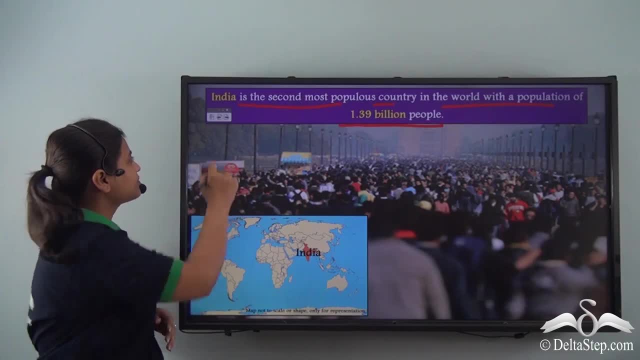 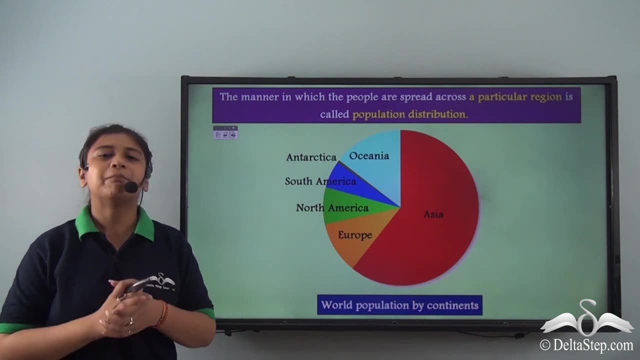 in the world with a population of 1.39 billion, so population is not equally spread across the world. people are unevenly spread across the world. there are some places that are highly populated. well, there are some places who has a low population? for example, countries like India are highly. 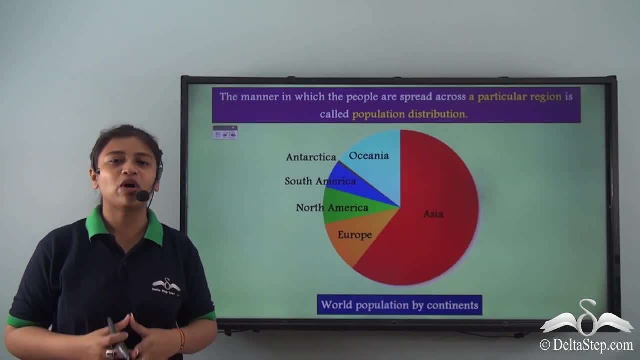 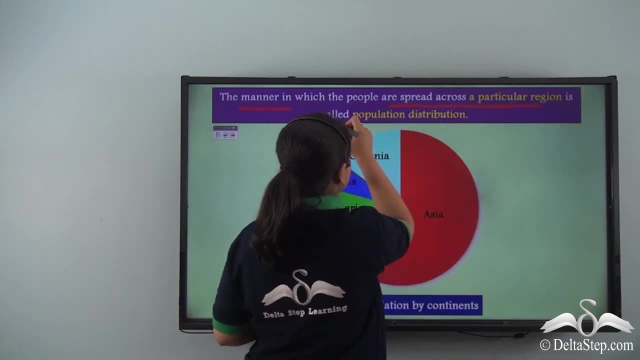 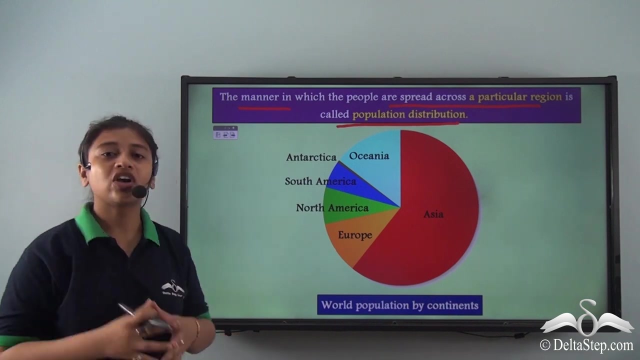 populated, while countries like Canada are less populated. so we can say that the manner in which people are spread across a particular region is different, and this is known as population distribution. now, if we consider the continents of the world, we know that there are seven continents, out of which 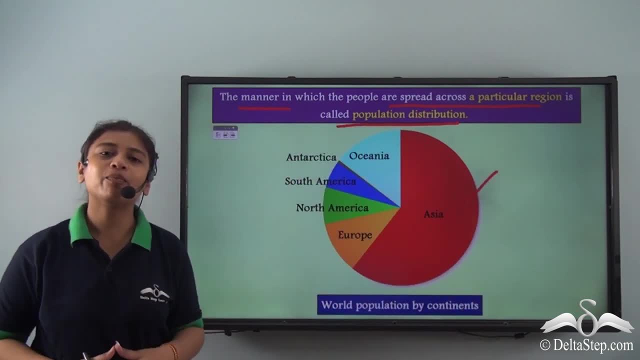 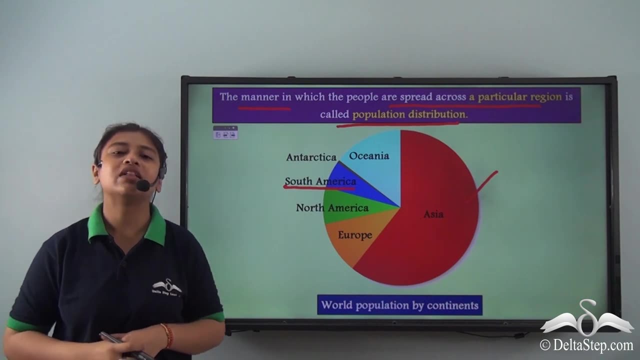 Asia is most populated among all the other continents, while South America is least populated among all the other seven continents. however, we have not taken Antarctica into consideration, as there are no permanent inhabitants. so we can say that the population distribution of the world is less than the population of the world. 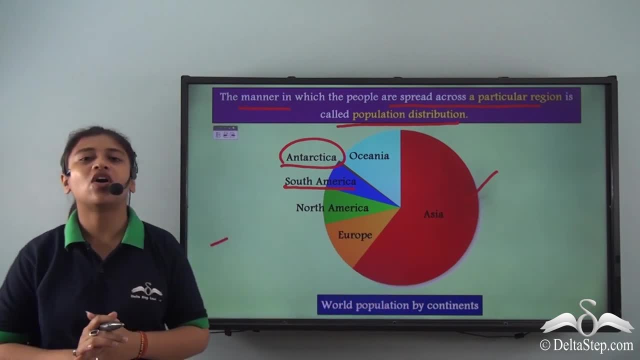 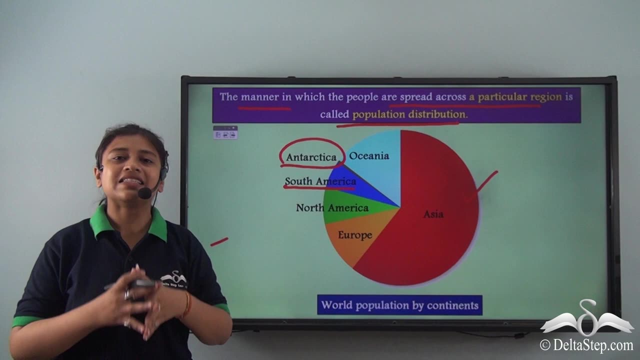 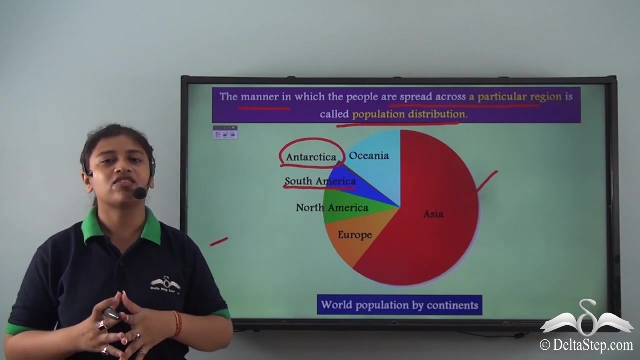 so Asias, that lies almost in the northern hemisphere and entirely in the eastern hemisphere, is most populated continent of the world, while South America, that lies in the Western hemisphere, completely and almost in the Southern hemisphere, is least populated. this only means that the population distribution is uneven across the world. 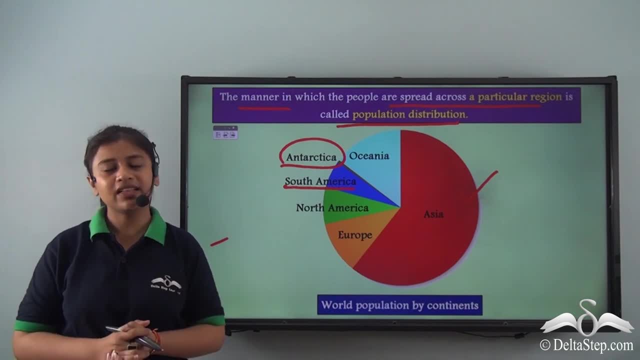 people are unevenly distributed across the world. there are places that has a high population and then there are places that has a low population. So in this lesson we were able to understand the meaning of population and population dynamics. Now, population dynamics is the study of how and why a population changes in size, structure and composition. 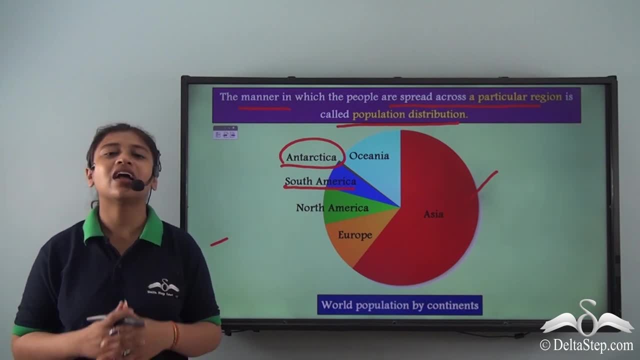 over time and space. We further understood that, among the population, people who are skilled and who are professionals in their own field are considered to be the most important resource of the country and therefore they are known as human resource. The human resource is important for any country as it helps in the continuous supply of labour, which helps in the overall 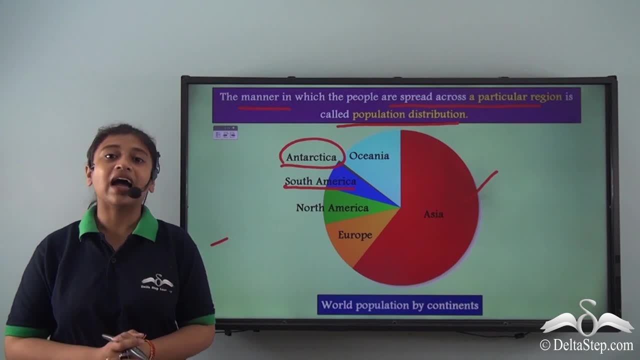 development of the country. We further understood that people are not equally distributed across the world and we further understood that the population distribution is uneven across the world. In our next lesson we will understand the meaning of population density. We will understand the difference between population and population dynamics.